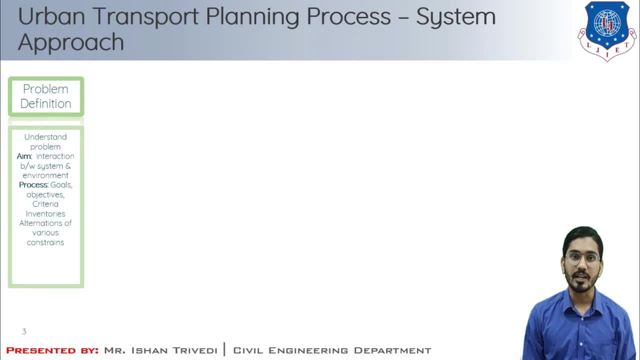 define the interface between the system and its environment. Here this system is nothing but various elements or factors of any city or a town. These are goals, objective criteria and standard set for particular plan. Here the inventory is done, like land use, employment, transportation, supply, transportation network, travel demand and so on. These type of study. 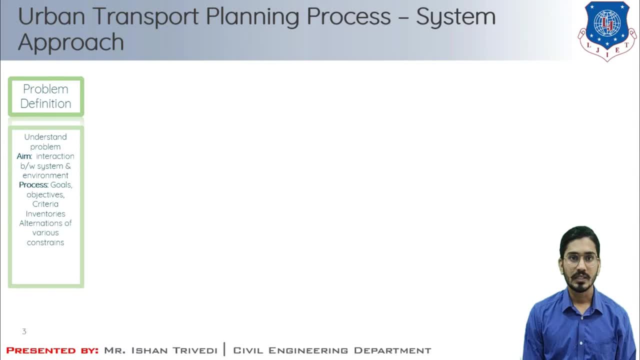 are carried out in this problem definition, The planner is forced to find the alternative means to solve Re Ranger's problem. Thus, constraints like finance politics acceptable to the service, to non car owner as well. In addition, certain financial and political pressures are there and exceptionally, 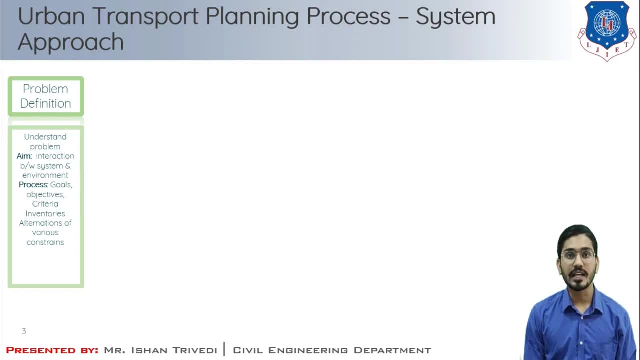 different kinds of alternatives are to be known, So not just know-it-all ones. so also to save our money. This is only exception factor of kind, or because these lowest quality solutions cant be bought to retail business, so most people buy a car for cheaper price. 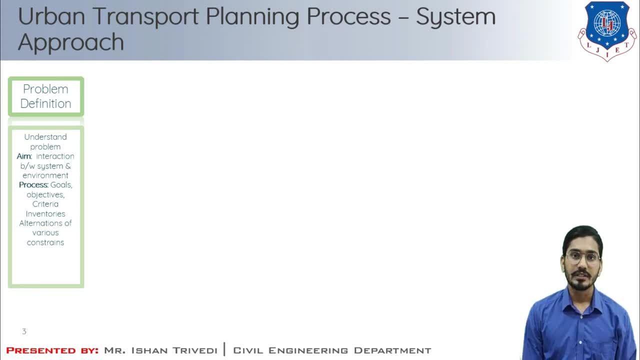 So they have to find out various alternatives while determining these problems. Next is solution generation. I mean cause generated, various parameters while asking the same question: cause buying a car is necessary? The aim of this stage is to generate the number of solution that satisfy the previously established objective in the problem. 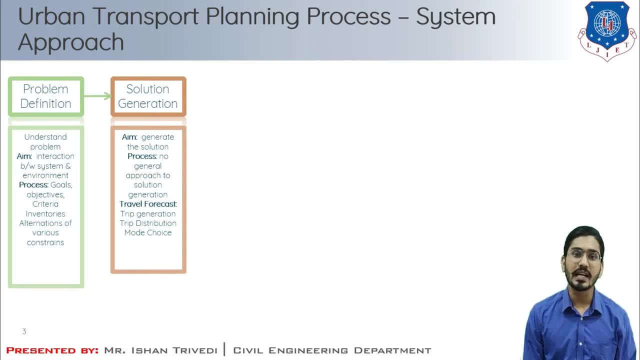 definition and to a greater or lesser degree, and which do not violate those constraints that I have discussed in problem definition. those constraints are again, I am telling you, those constraints are finance politics and acceptable services to non car owners. there is no general approach to solution generation and in this solution generation, travel forecasting is been done. these includes 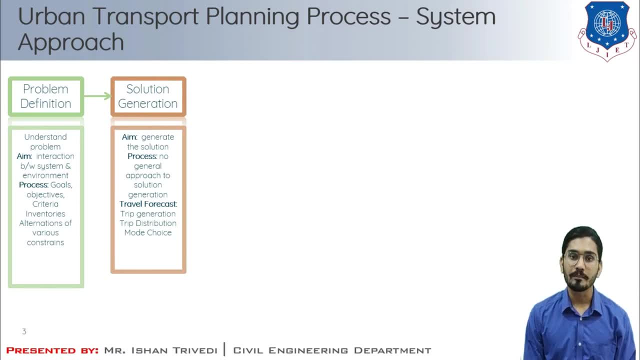 by trip generation, trip distribution and more choice. next is solution analysis. in this stage, each alternative solution that has generated during the solution generation process is called solution analysis. in this stage, each alternative solution that has generated during the stage two is been studied a by its operating characteristics and behavior. 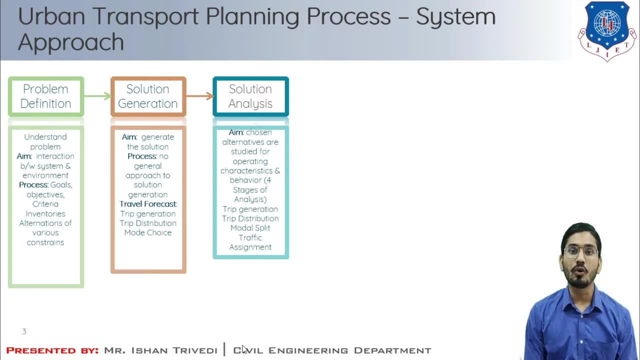 this prediction is done through a fourth phase of process, this consisting of trip generation analysis, trip distribution analysis, traffic assignment analysis and, at last, model split analysis. this will be discussed in detail in further more chapters. so what you have to remember here, whatever the problem has been found out, 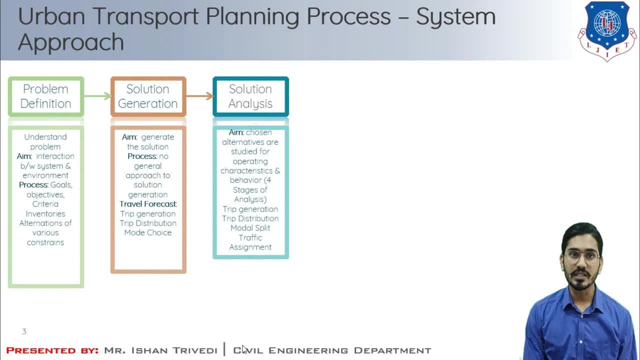 we have to find out the alternative, then solution generation, and based on those solution generation, we have to find out the solution analysis. and here this solution analysis is being divided in four stages. again, I am repeating: these stages are of trip generation analysis, trip distribution analysis, traffic assignment analysis and, at last, model split analysis. 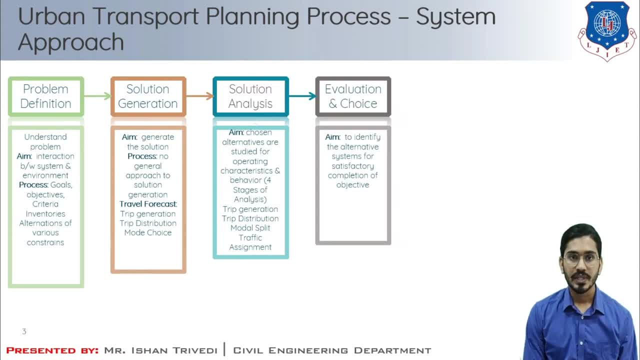 next is evaluation, evaluation and choices. the purpose of this stage is to identify the alternative system that satisfy the objective. to a great extent. these objective are made in the problem definition and based on that I have derived the ample of solution and I analyze those solutions as well. now what I am doing, and doing the evaluation. 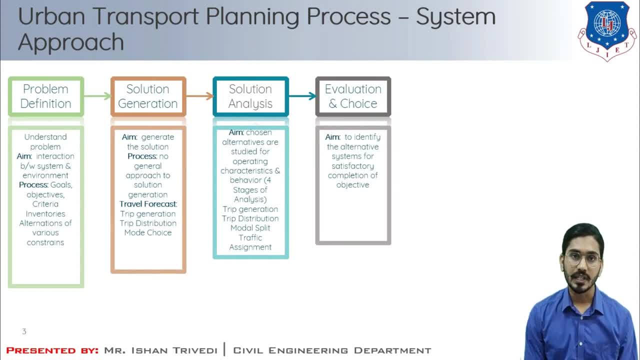 of whatever the choice and alternative that I have, clear and based on the system, I will put appropriate solution to the system. Next is recommended plan. Stage 4 ultimately gives us the most effective plan which can be recommended as a final optimum plan. So, whatever the study has been carried out, now I will going to implement, and for that, 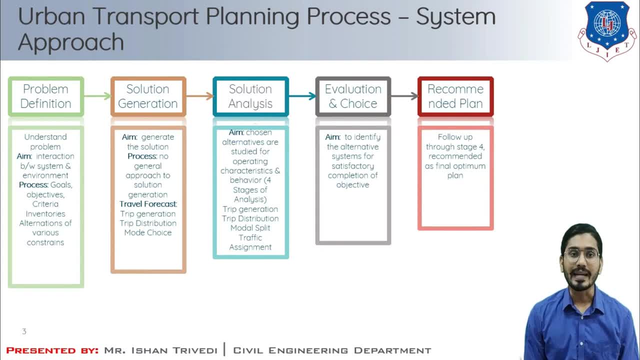 I before that what I have to do, I have to precede my activity, that is of evaluation, and I will take the recommendation based on the evaluation that I have done in the system. After this, the last, is the implementation of the plan. The final optimum plan for the horizontal year identified in the last stage requires: 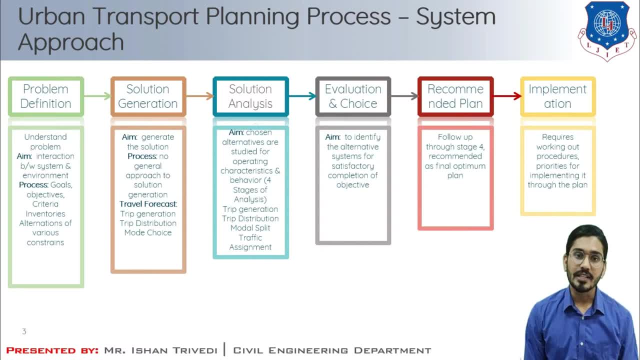 working out the procedures, priorities or implementing it through a plan. So, whatever the recommendation has been done, it will be implied In the evaluation and final stage is to implement in the real practices, based on the requirement, priority and the procedure that we require to follow to implement certain things. 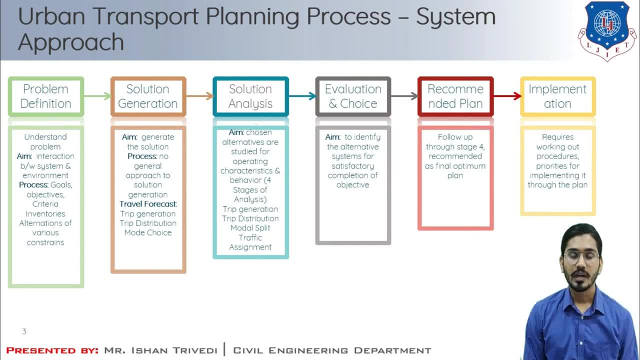 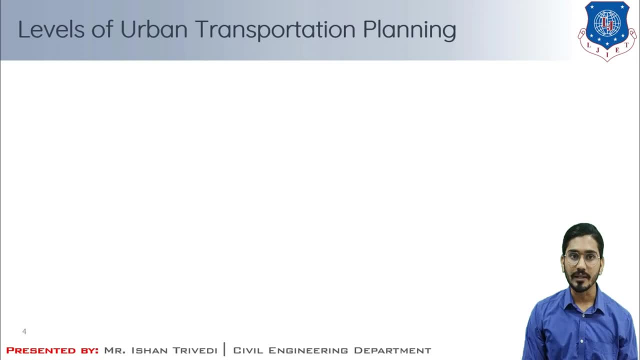 So these are the systematic approach of urban transportation planning. Next is levels of urban transportation plan. The transportation planning studies are carried out at number of stages, At number of levels, having different type of details and decision to be accounted. The planning or design agency and the team also changes from level to level. 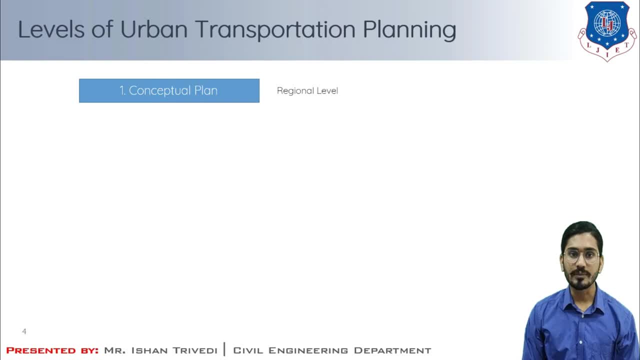 So these levels are: first is conceptual plan. It has been done at regional level, Based on conceptual plan. the outline plan is been prepared, which is at sectoral level. All the planning is done at regional level Based on conceptual plan. the outline plan is been prepared, which is at sectoral level. 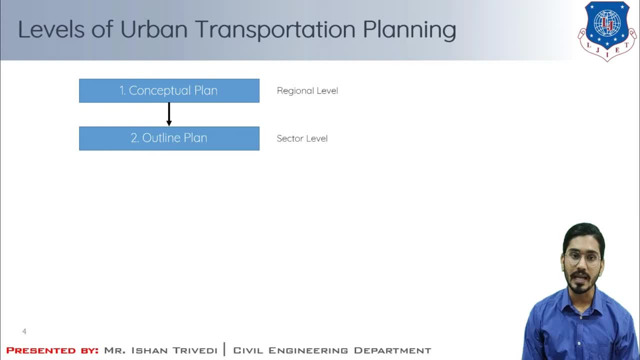 All the feedback has been received from conceptual plan is been implemented in outline plan. So the feedback of the conceptual plan to a broader extent is been implemented in outline plan. Based on outline plan, the master plan at district level is been prepared. Then a statutory or local plan, or you can say advisory plan, is been done at local level. 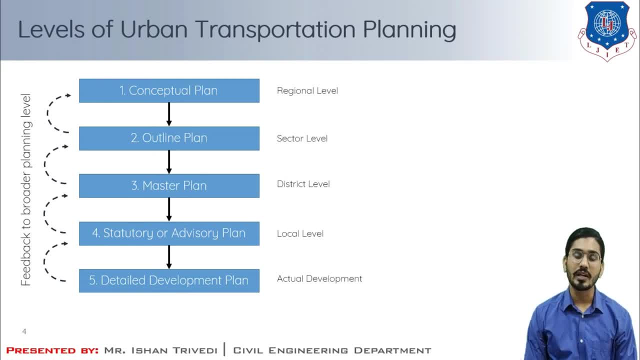 Then a statutory or local plan of city level And then a code plan is applied based on actual development. So after this level development plan has been implemented, it has got 4 levels. the entire plan is indeed aire focused property reason. Now the'vocum here is how theczylial plan works based on this in the perhaps ^^. 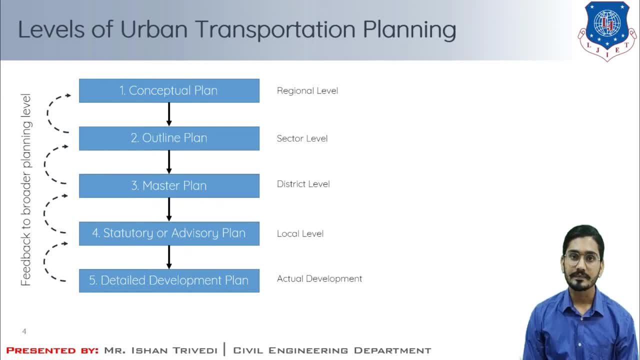 detail. development plan is been implemented based on actual development. So, whatever the plan is been implemented, it is based on preceding plan or the preceding plan area focus. So whatever we have done, For example for statutory plan, what I'll do, I will take a reference of the particular söyled area focus. 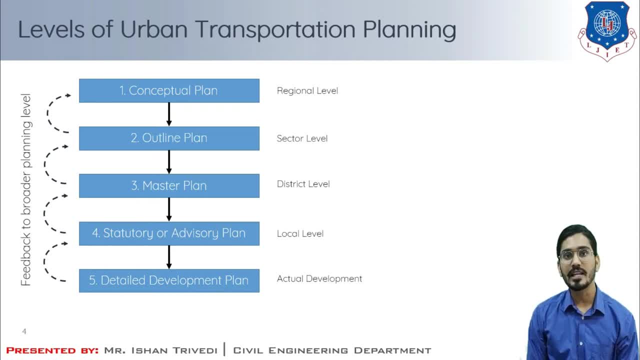 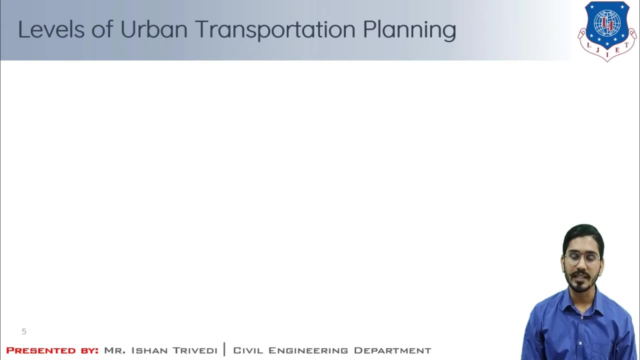 Why I I have adopted it as a new plan. Then within this, that is the popular development plan of master plan, and based on that, the statutory plan or advisory plan is been done. So let us discuss these things in detail Now let us study these levels of urban transportation planning in detail. 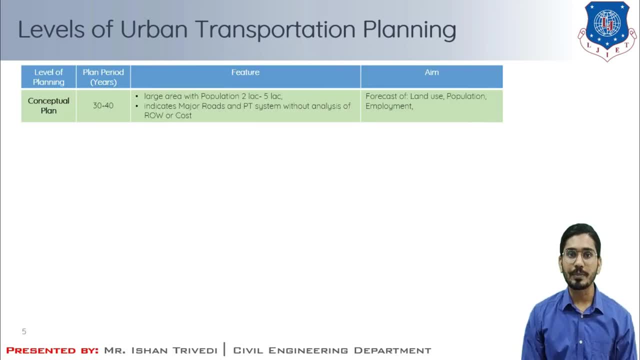 First is conceptual plan. The conceptual plan is prepared for the broadest level of planning where the planning period is large, After it has been kept, up to 30 to 40 years, which caters very large area with the population ranging from 2 lakh to 5 lakh. 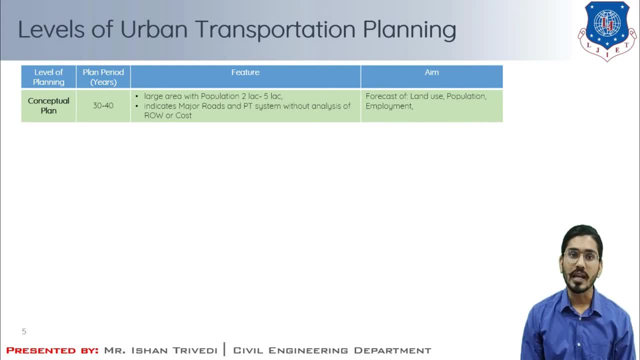 The aim is to make forecast for land use, population employment and consider the economic status of the area. It indicates major roads and public transport system for the whole area, without analysis of rent. Next is outline plan. Outline plan is developed keeping in the view of conceptual plan, as I discussed in earlier. 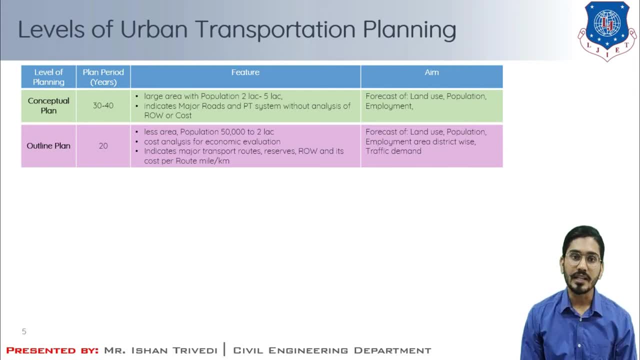 listing. The planning period is about 20 years and it has lesser area and you can say the population is around 50,000 to 2 lakh. It involves the forecast of land use, population, employment area, district by district. When I am talking about the traffic demand, the benefit to cost analysis is used for the 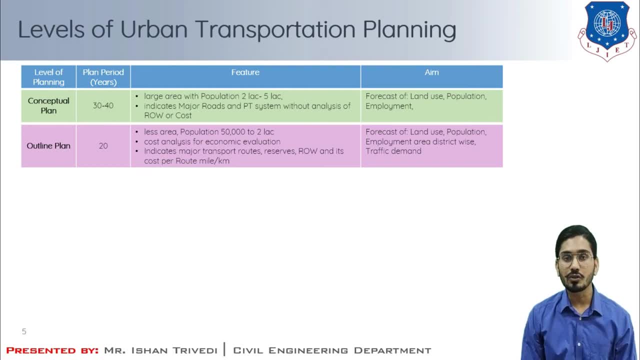 economic evaluation. This benefit to cost is based on the socio-economic parameters, and social welfare is been considered in the benefit cost analysis, Whether the cost which are used for the developing the town is fruitful or not. So for that, what we have to consider is the cost analysis. 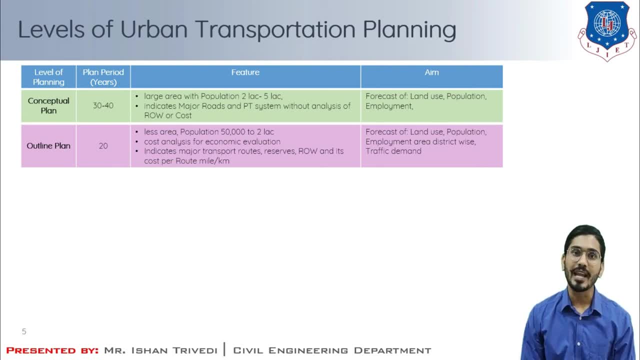 So for that, what we have to consider is the cost analysis. So to exam that, what we have to do, we have to analyze the benefit to cost analysis in this transport planning process. and that is nothing but an economical evaluation. It indicates the major transport routes, reserves, right of ways and cost per route of één. 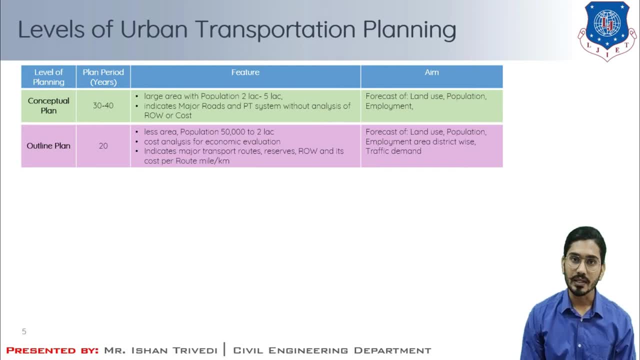 mile is worth out. Next is master plan. Master Plan is developed keeping in the view of the objective of outline. Flagging needs to be in keeping with the objective of outline plan. The planning period is smaller, about 20 years. It has lesser area and population district, up to 5000 to 10000. 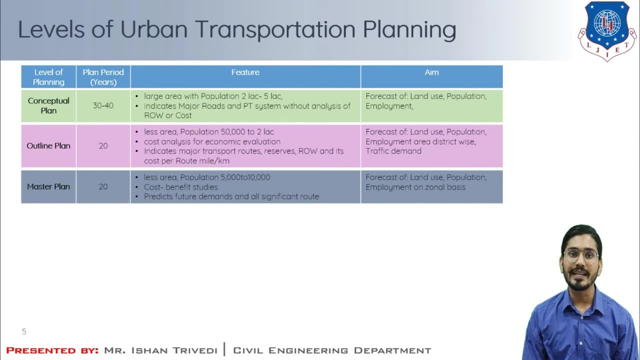 Here the population, land use, employment is predicted on a zonal basis. Earlier it was district wise, now here it is based on zonal basis and the detailed cost benefit studies are carried out in this master plan. It predicts the future demands and all the significant routes which are established in. 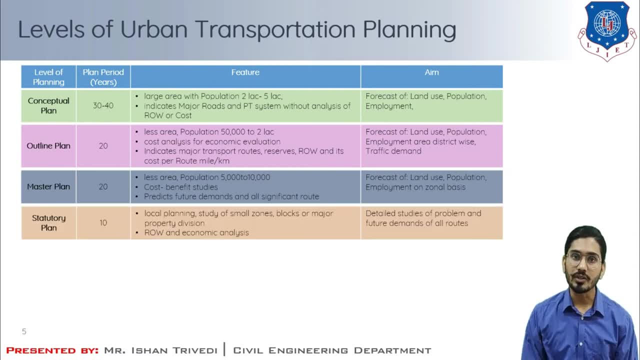 future. Next is statutory plan. Statutory plan here scattering the objectives of previous level of master plan. This stage involves the local planning. The planning period is 10 years. The study areas are in small zones, or you can say blocks, or major property division. 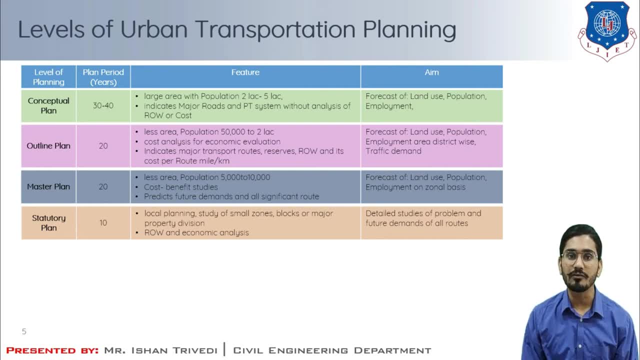 Detailed studies are undertaken in the view of problem and the future demand of all the significant routes, which are undertaken on comprehensive basis. The detailed implementation plans are work out here and rigid write off way and economic analysis are done. Last is detailed plan. Detailed plan preparation involves various things, for example, formation of detailed land. 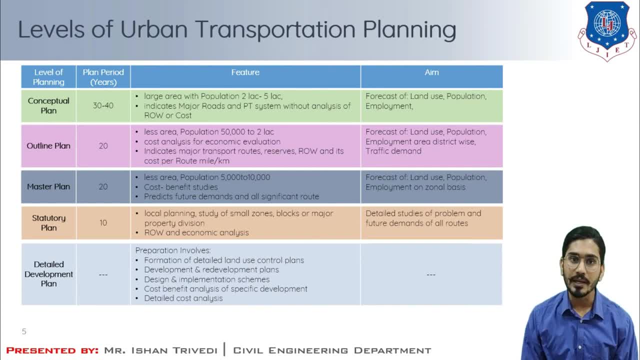 use control plan, development and redevelopment plan, design and implementation schemes, cost benefit analysis of specific development proposal and detailed cost analysis. So these are the levels of urban transportation plan. I hope you have understood. Now let us study the basic structure of transportation system. 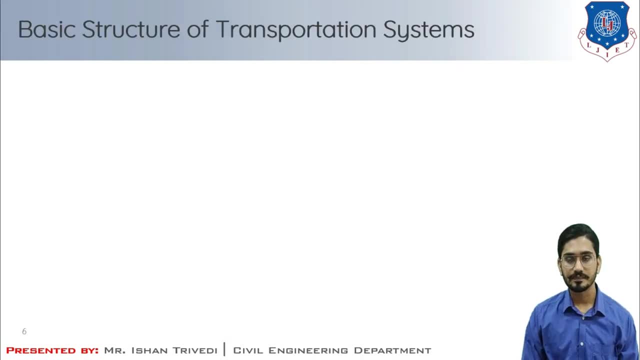 When I categorise this urban transportation system, it will be in two parts, that is, motorized transportation and non-motorized transportation. Non-motorized and motorized transportation are categorized in two categories, ie passenger transport, goods transport. When I further categorise this urban transport in to two categories, ie России transportation. 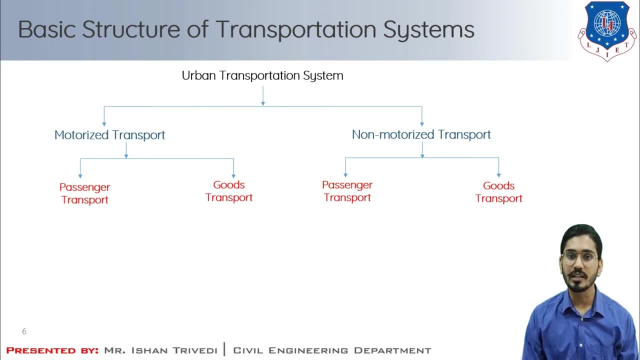 this non-motorized transportation system, in particularly passenger transport and goods transport. these are walk, bicycle, cycle rickshaw. in passenger transport and for goods transport it is hand cart and animal drawn cart. Furthermore, if I classify the motorized transport in terms of passenger transport, there are: 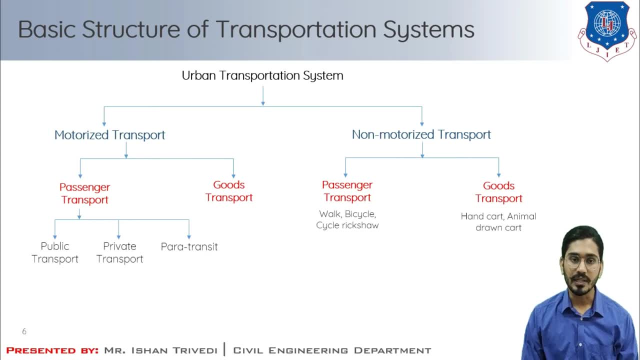 three major classification: First is public transport, second is private transport and third is paratransit. The type of vehicle in this three category are bus, train, metro, monorail and LRT for public transportation. For private transportation there are cars, van, motorcycle and so on, and for paratransit. 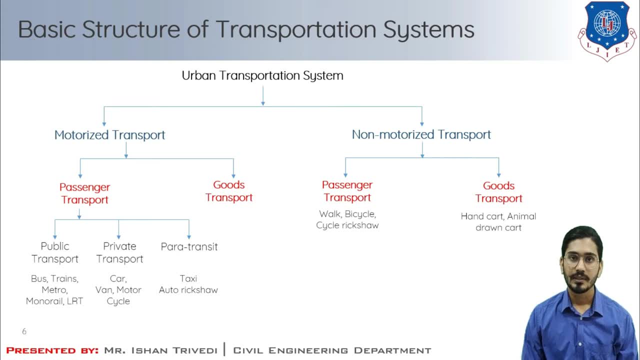 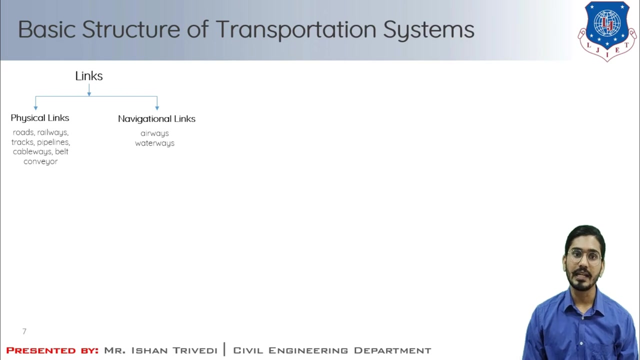 it is taxi and auto rickshaw, or you can say it is of intermediate public transportation. If I am talking about goods transport, there are truck, tempo van and cart. so these are the basic structure of transportation system. Furthermore, if I am talking about the links, then there are physical links and navigational 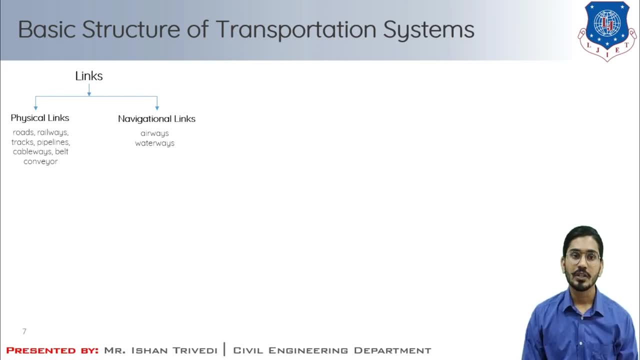 links. Physical links are related to road, railway tracks, pipeline, cableway, belt, conveyor and navigational links are related to vehicle. These links are airways and waterways, If these links are categorized in terms of means of movement of person and the goods. 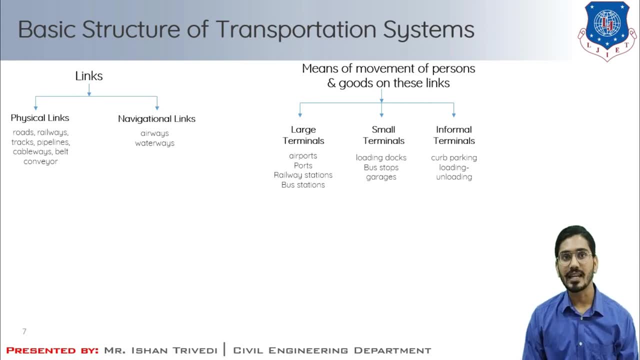 then there are three categories. these categories are large terminal, small terminal and informal terminals. If I am talking about large terminal, these are airports, ports, railway station and bus station. Then small terminal are of loading docks, bus stops and garages. For informal terminals, these are kerb parking, loading and unloading areas. 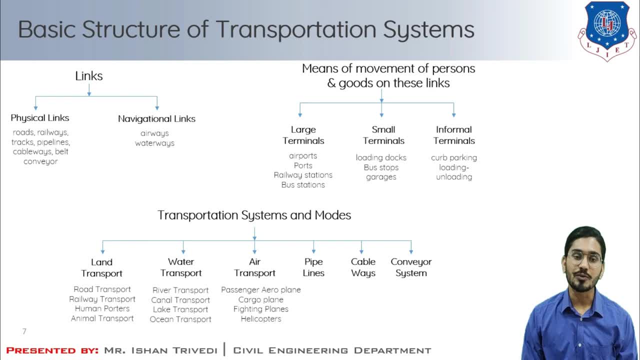 Furthermore, if I am talking about transportation system and their various modes, then there are Land transport, Water transport, Air transport, pipelines, cableways and conveyor systems. Land transport are of road transport, railway transport, human porters and animal transport. If I am talking about water transport, then the modes are river transport, canal transport, lake transport and ocean transport. 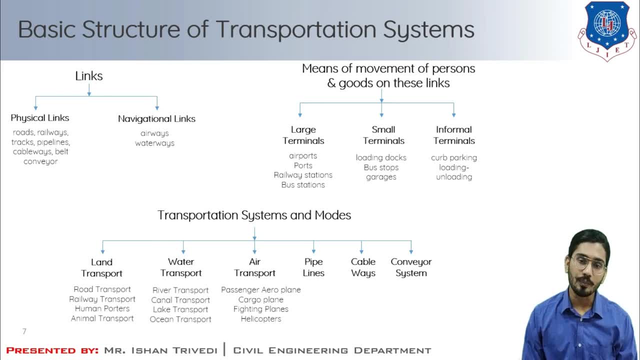 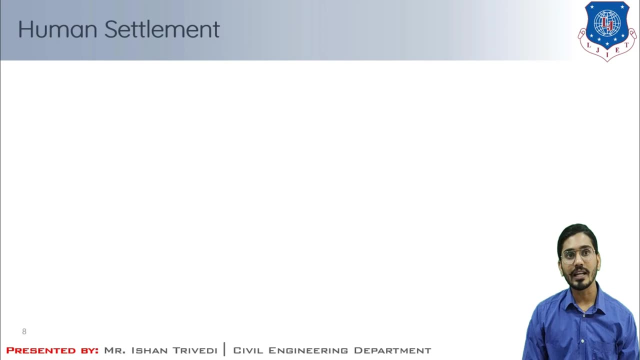 Then air transport includes passenger aeroplane, cargo plane, fighting plane and helicopters. So these are the basic structure of transportation system. Now understand the theory that is human settlement. Human settlement are broadly classified in two parts, that is, rural area and the urban area. 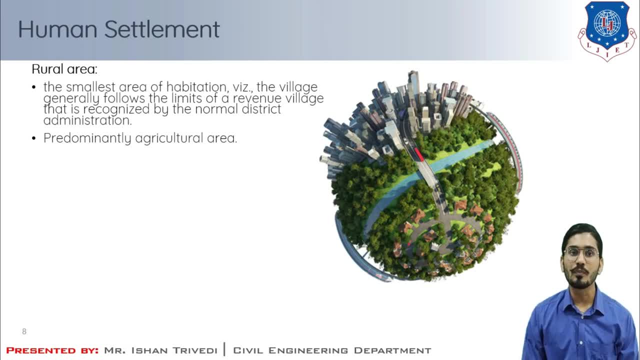 If I am talking about the rural area, then it is a smallest area of habitation, or you can say a village which generally follows the limit of a revenue village that is recognized by the normal district administration, Or you can say it is nearly an agriculture area. 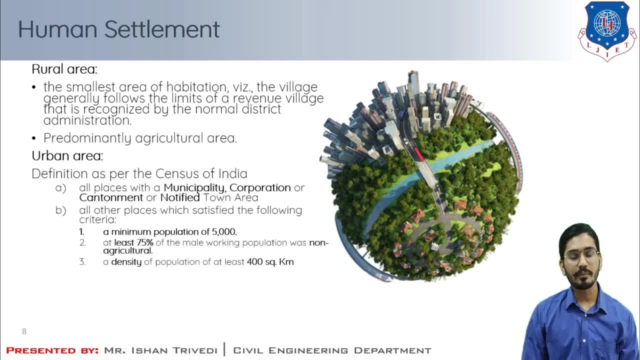 Now, second is urban area. Urban area has been classified as per the census definition of India. There are two categories which defines the urban area. These two categories are: First among these are All the places within a municipality corporation Or a cantonment or notifed town. area means a city which has a local municipality or corporation. then you can say it is an urban area. 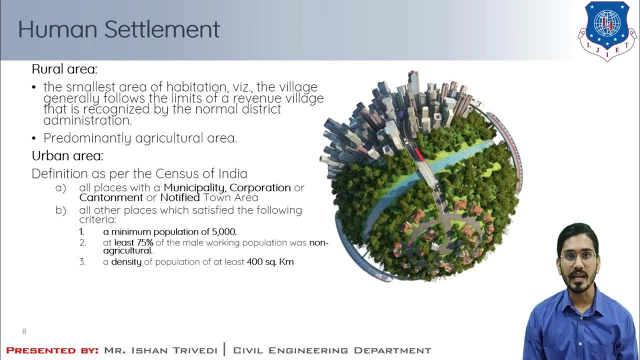 Ahmedabad has its own municipality, so Ahmedabad is an urban area. Another definition is All other places which satisfy the three main criteria. Among these, first is A minimum population of an area has to be 5000.. At least 75% of male working in non agriculture activities. 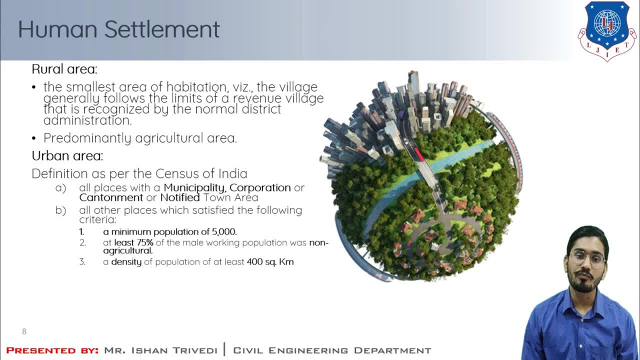 And, at last, a density of population is 400 per square kilometer. If any place is not a community, then it is a sub-district. If any place is not a community, then it is a sub-district. If any place is not a community, then it is a sub-district. 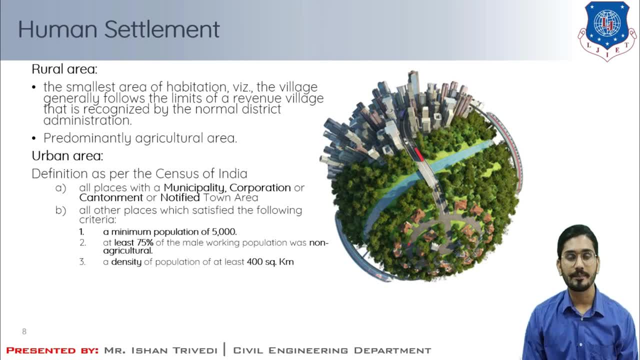 If this or any area satisfies all these three criteria, then you can call it an urban area. This is nothing but the definition of a statutory town as per the Census of India. This is nothing but the definition of a statutory town as per the Census of India. 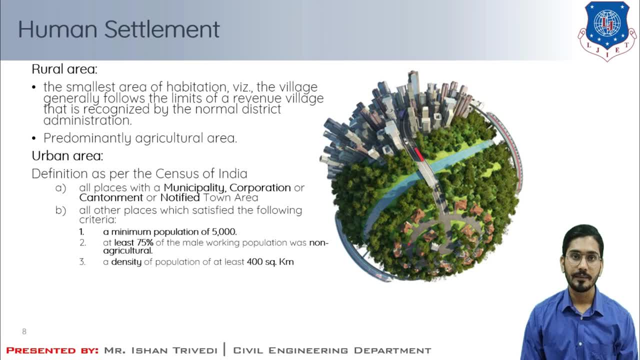 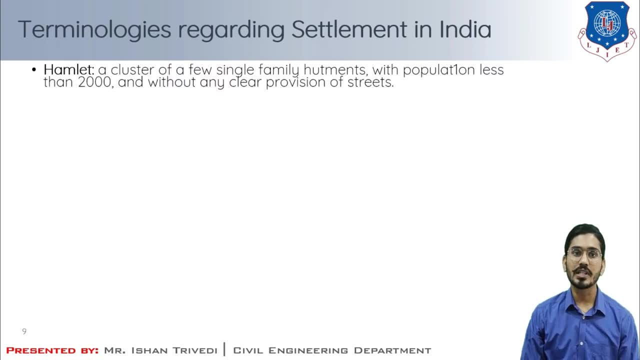 Furthermore, let us understand few terms in brief. Furthermore, let us understand few terms in brief. First is Hamlet. It denotes a cluster of a few single families, hut-men, with the population less than 2000 humans and more than 2000 workers. 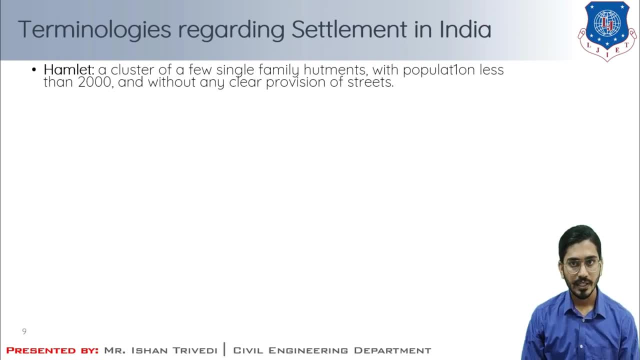 and without any clear provision of street. In Gujarati it is been known as a Para area or Para Vista. Next is Village. Village consists of a number of dwelling unit with definite street pattern, usually with a population between 2000 to 20000 and with basic amenities like primary school. 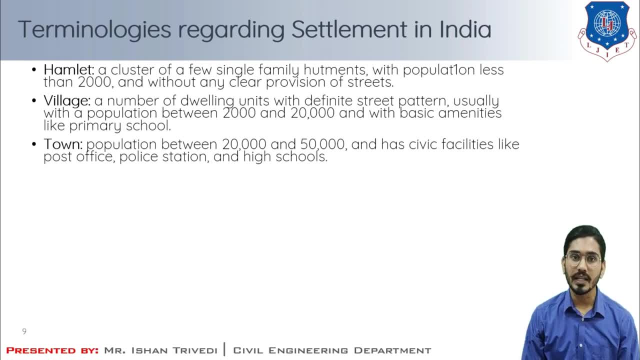 Next is Town. Town has a population between 20000 to 50000 and have basic civic facilities like post office, police station and high schools. Next is a City. A city has a population between 50000 to 1 lakh and will have most of the civic amenities. 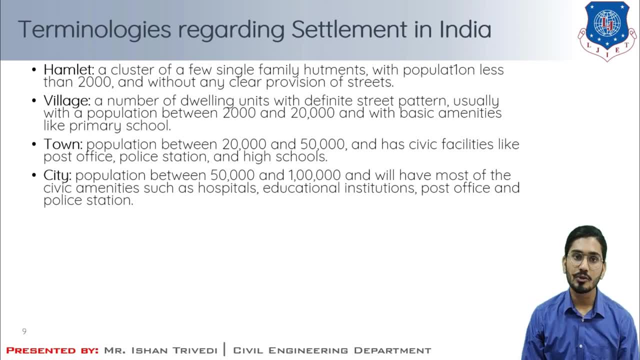 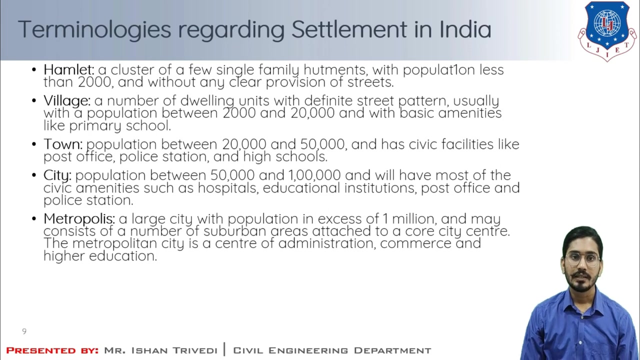 such as hospital, educational institute, post office and police station. Then Metropolitan. It is a large city area with a population in excess of 1 million, and may consist of a number of sub-urban areas attached to a core city centre. The Metropolitan city is a centre of administration, commerce and higher education. Then, at last, Megapolis. Megapolis occurs when two or more metropolitan cities are connected to each other. Megapolis is the centre of urban development. The metropolitan cities lies adjacent to each other, forming a continuous urban agglomeration. Now, if I classify these all the towns in terms of population, based on URDPFI guidelines, 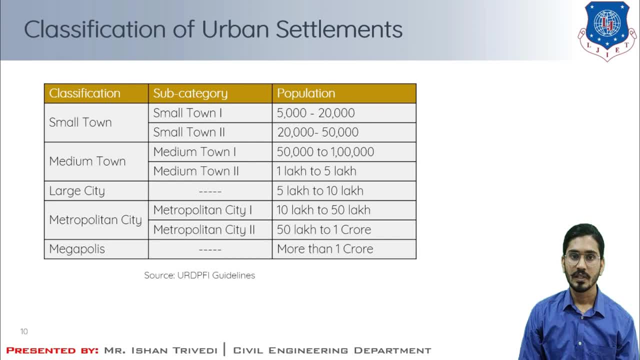 these classifications are: for small town. the sub-category is divided into two parts, that is, small town 1 and small town 2.. For small town 1, or you can say a statutory town, the sub-category is divided into two parts, that is, small town 1 and small town 2.. 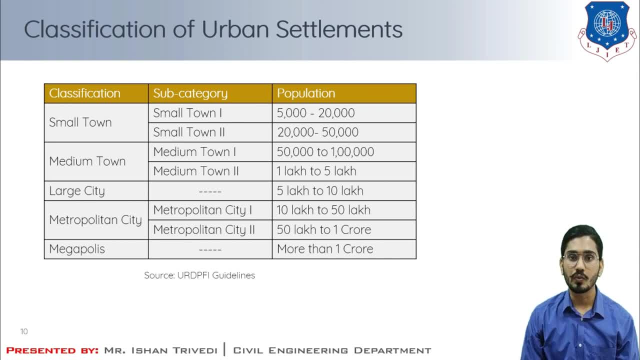 For small town 1, or you can say a statutory town, The population is of 5000 to 20000, and for small two, the population is of 20000 to 50000.. In medium town 1, the population is also further 5k to 1k. 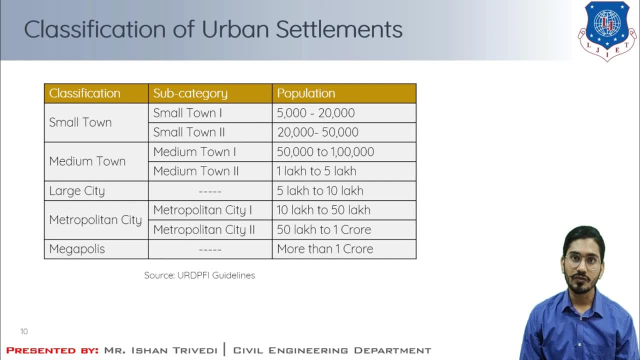 For medium town 2, it is also further classified in two and for medium town 2 it is the same I was saying from: 1. For Large city, the population lies between 5k to 10k. For large city the population is also same. I was saying 5k to Mail Def azar ca API.